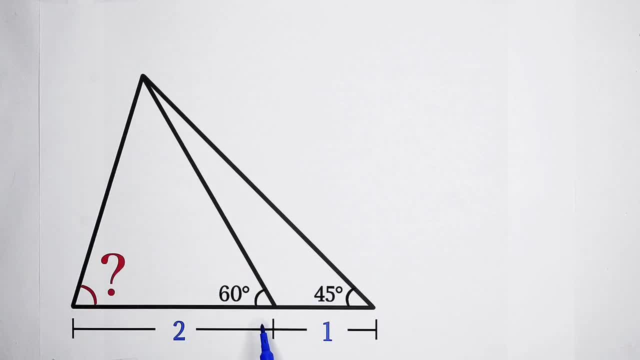 This is a triangle and this angle is 60 degrees. This angle is 45 degrees. The length of this segment is 2, and the length of this segment is 1.. Question: How many degrees does this angle have? We have to solve for the value of an angle. 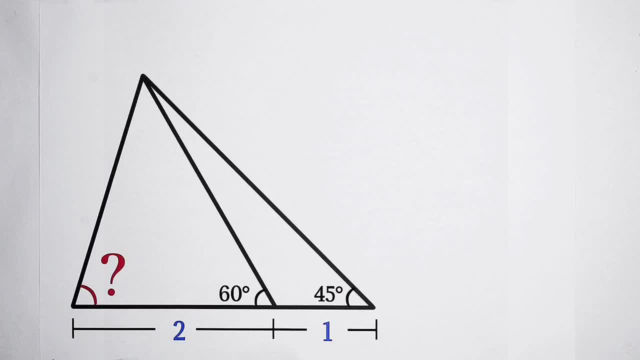 So for the length, we just have to consider their relationships. However, first take a look at these two angles- 60..45.. They're both nice angles. Let's start from the 60 degrees Yearsly. if we see 60 degrees, we have to consider a right triangle which contains: 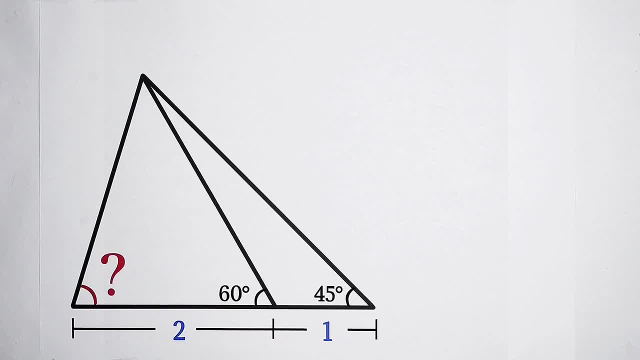 it. Our problem is how to construct a right triangle from here or from here. For construction on a right triangle triangle, we have to make the perpendicular of ac through the point b. since the length of bd is 2, we can calculate the length of ed directly by using cosine of 60 degrees. 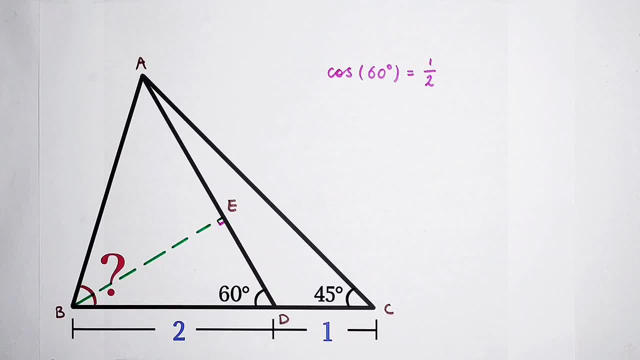 is one half. firstly, we can solve for the length of d? e cosine of 60 degrees is bd divided by d? e. so d e is cosine of 60 degrees, then times b d, that means it is 1 over 2. then times the length of bd. 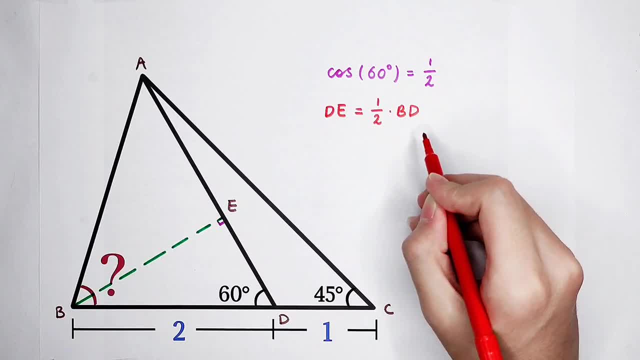 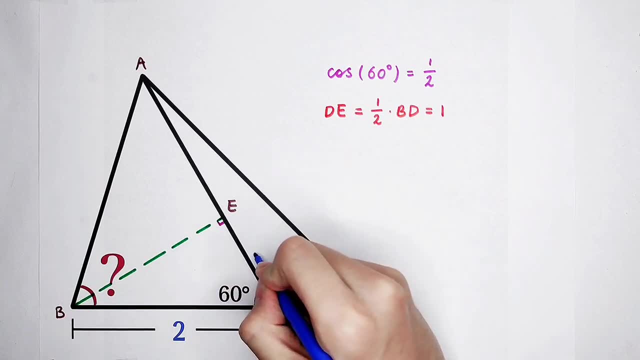 since the length of bd is 2, so d e is 1, so the length of d e is 1. we've labeled it. and then we have to consider this angle, 45 degrees, and maybe you have noticed that the length of cd is also one. so if we connect c and e we can get an isosceles triangle. go back. 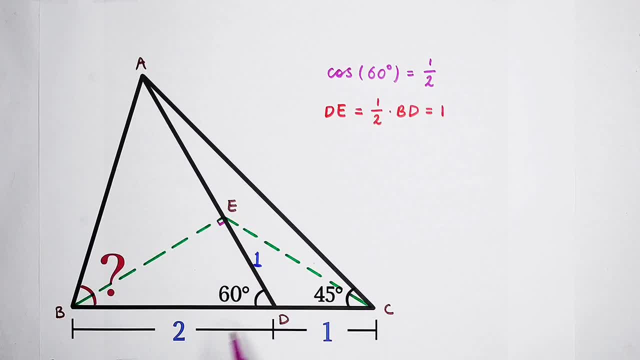 to this triangle. the angle edb is 60 degrees is known, and the angle dbe can also be solved. 90 degrees minus 60 degrees is 30 degrees, since we have to solve for the angle abd and the section of it dbe has been solved, so now we have only to consider solving. 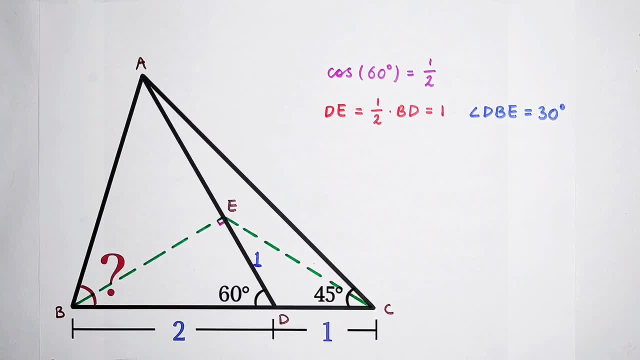 the angle a, b, e, and how many degrees is this angle? we connected c and e and the triangle cd- e is an isosceles triangle. since cd is equal to d? e, they're both one. now, according to exterior angle theorem of a triangle, an exterior angle of a triangle is equal to the sum. 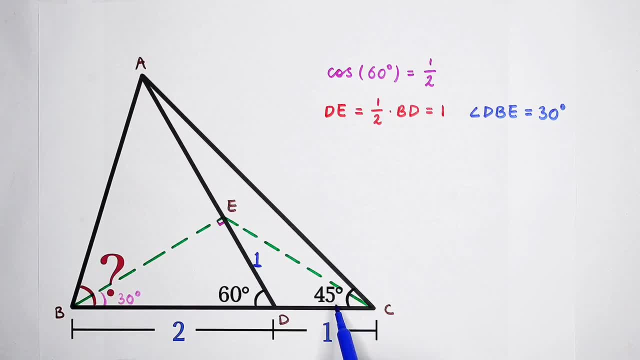 of the two interior angles that are not adjacent to it. so that means the angle bde is equal to sum of the angle cd and the angle dce. these two angles are equal and their sum is 60 degrees, so each of them should be 30 degrees. this angle is 30 degrees. 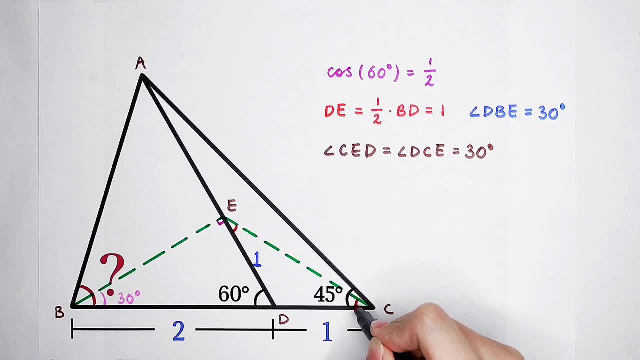 and this angle is 30 degrees as well. most of you have found out that the angle cbe is equal to the angle bce. they're both 30 degrees. so what does it mean? it means the triangle bec is an isosceles triangle as well. 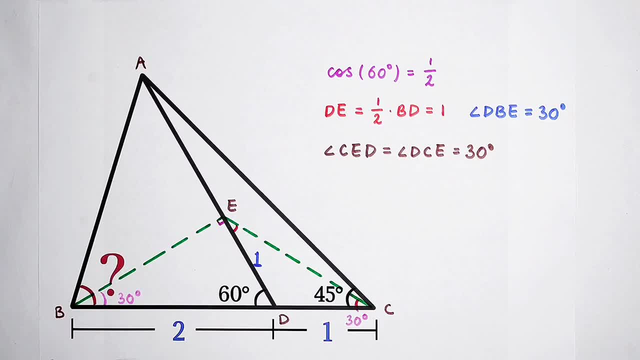 just like this triangle. if a triangle is an isosceles triangle and then be is equal to ce, they have the same length. we have already analyzed these two triangles. we only lack this one. now try analyzing this triangle, the triangle aec. is it also an isosceles? 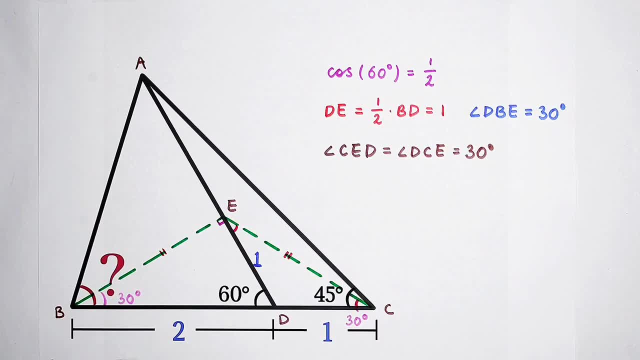 triangle. we don't know, maybe, but we're not sure. the angle acb is 45 degrees and the angle ecb is 30 degrees. so the angle ace, of course it is 45. then minus 30, it is 15 degrees, again according to exterior angle theorem of a triangle. 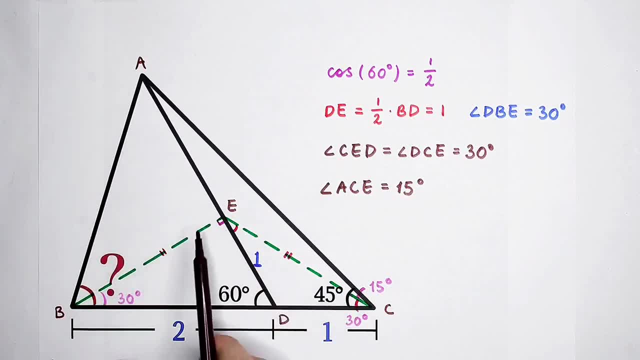 the angle cae. then plus the angle ace is equal to the angle c ed. since the angle ced is 30 degrees and the angle ace is 15 degrees, so the angle cae is equal to 13. then minus 15 is 15 degrees. 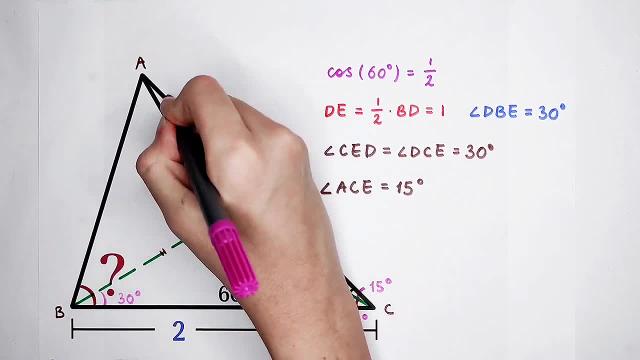 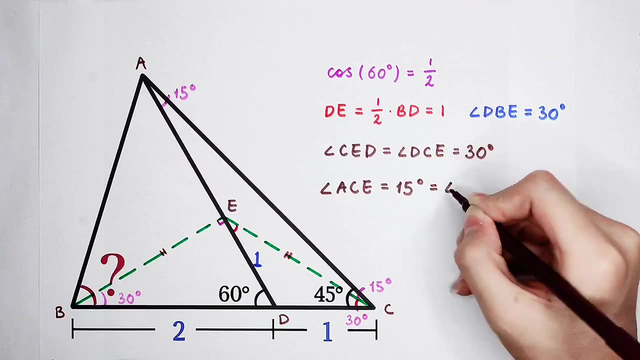 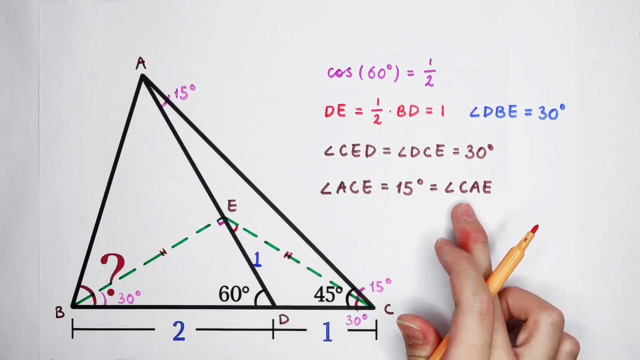 so the angle CAE is also 15 degrees. So these two angles have the same degrees: The angle ACE and the angle CAE. what can we get if they are equal? Of course, this triangle CAE is also an isosceles triangle. If this triangle is an isosceles triangle, 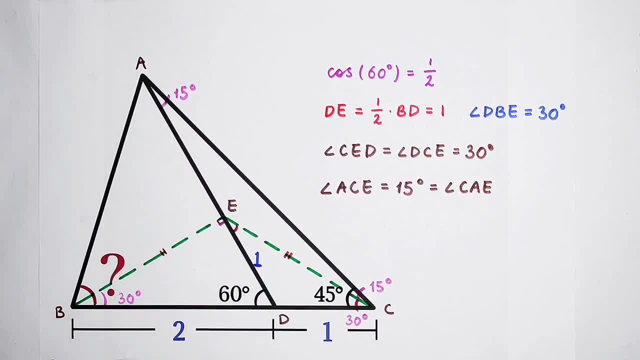 then CE is equal to AE, Since we got the triangle BEC is an isosceles triangle, so BE is equal to CE. And the triangle CAE is also an isosceles triangle, So CE is also equal to AE. So that means AE is equal to BE. So this triangle, AEB is. 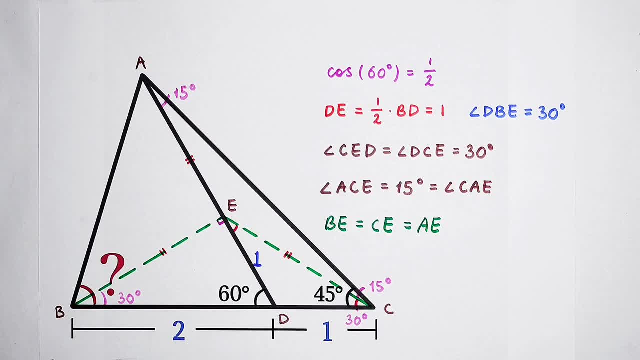 an isosceles triangle as well. Now question: Is it only an isosceles triangle? Are there any other characters? Have you noticed? The angle BED is a right triangle, So the angle BED is 90 degrees, So that means the